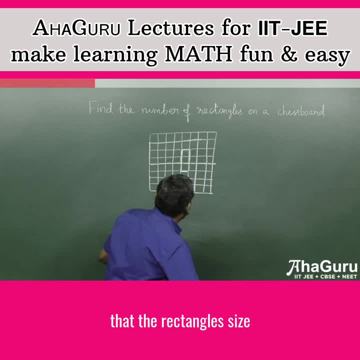 Okay, now, for example, you can say that the rectangles size. you can find the number of rectangles for each size. So, for example, if you say that, okay, let me take rectangles of width 1 and then find how many different possible rectangles are there. 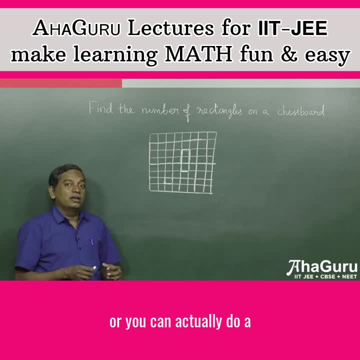 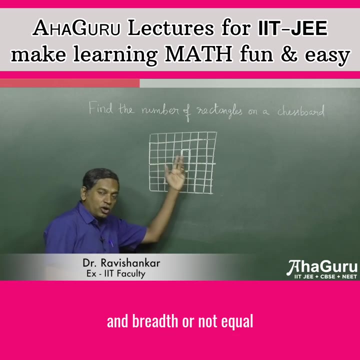 All such possible cases and add, Or you can actually do a much shorter approach. What is the shorter approach? Well, actually, if you want to form any rectangle on this chessboard, whether it's a rectangle where the length and breadth are not equal, or a square where the length and breadth are equal, 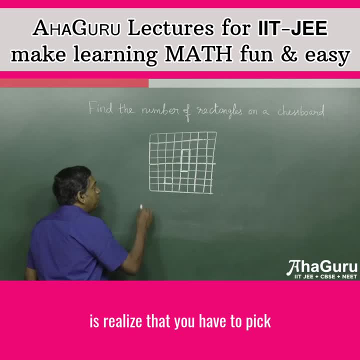 what you need to do is realize that you have to pick two vertical lines. Okay, for example, let's say I pick these, This vertical line and this vertical line. Okay, you can clearly see that I've picked these two and pick two horizontal lines. 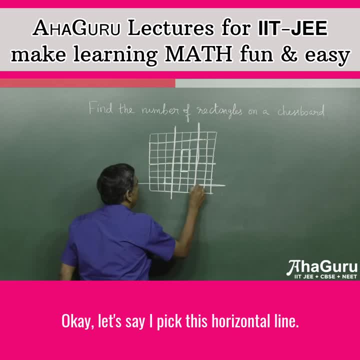 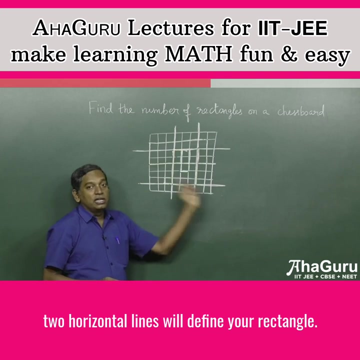 Okay, let's say I pick this horizontal line and this horizontal line. Now what you see is that these two vertical lines and the two horizontal lines together define the rectangle, which means the rectangle that I've picked just now is this rectangle. So what we have realized is that picking two vertical lines and two horizontal lines will define your rectangle. 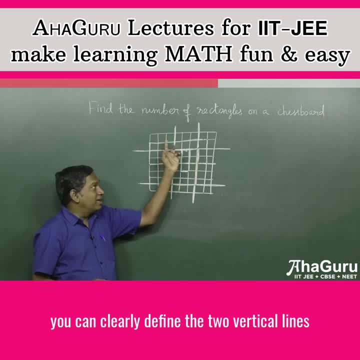 Try it For any rectangle. okay, you can clearly define the two vertical lines and the two horizontal lines and this is a unique mapping For every pair of vertical lines plus horizontal lines. you're going to have two vertical lines. You're going to have a unique rectangle. 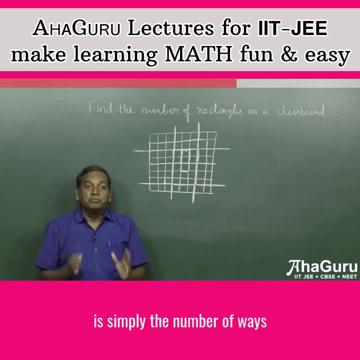 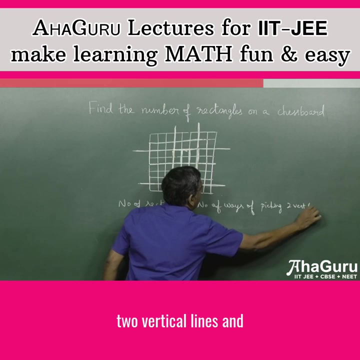 Well then, what does it mean? The number of rectangles is simply the number of ways of picking two vertical lines and two horizontal lines. So number of rectangles is number of ways of picking two vertical lines and two horizontal lines. Well, we know that the number of ways of picking